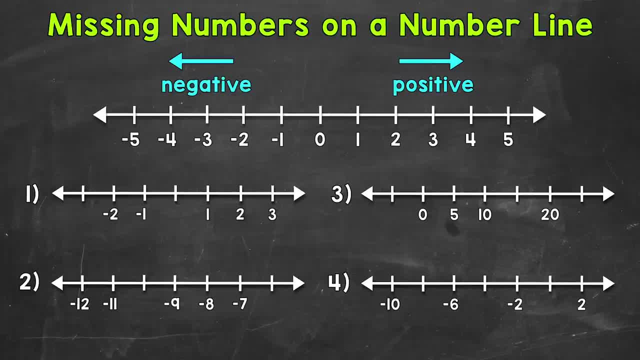 So we can see that we are counting by one. Once we figure that out, we can find the missing numbers. We can either count up or count down using that distance between numbers in order to find the missing numbers. So, for example, let's count down from three. 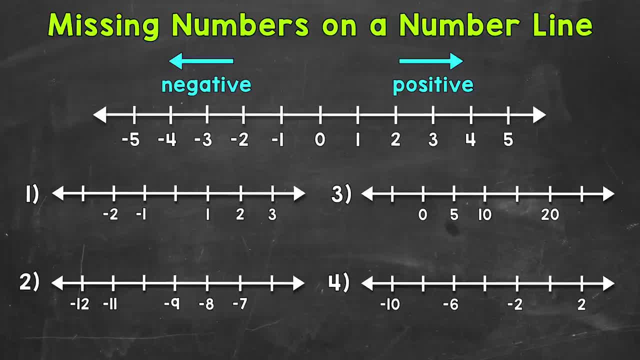 Because we know we're counting down by one, Three, two, one and then zero. So we have a zero for this missing number here. Let's continue to count down. Then we have negative one, negative two and then negative three. 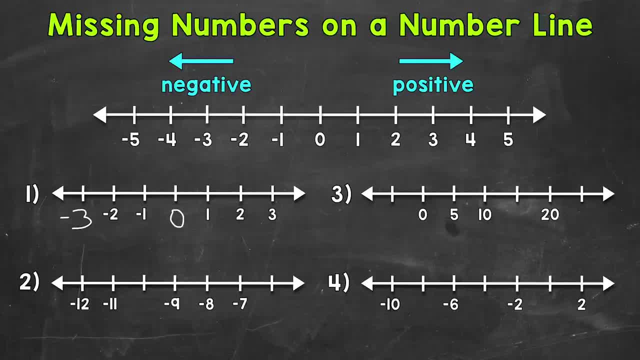 Once we have those missing numbers filled in, we can double check. So let's count up now and see if those missing numbers that we filled in are correct. So: negative three Negative three, negative two, negative one, zero, one, two, three. 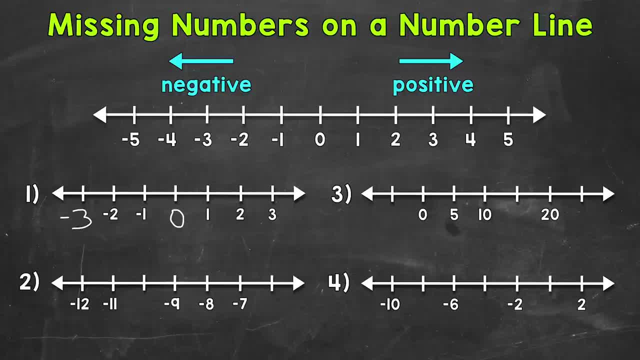 So those are the correct missing numbers. Let's try another one and move on to number two. So we're going to take a look at what we're given, Starting with negative twelve and then negative eleven, So we have a distance of one there. 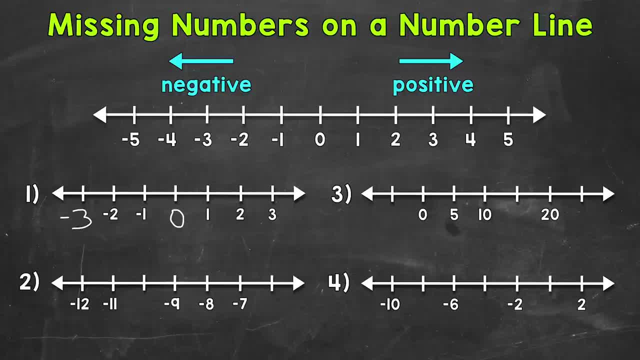 So those are the correct missing numbers. Let's try another one and move on to number two. So we're going to take a look at what we're given, Starting with negative twelve and then negative eleven, So we have a distance of one there. 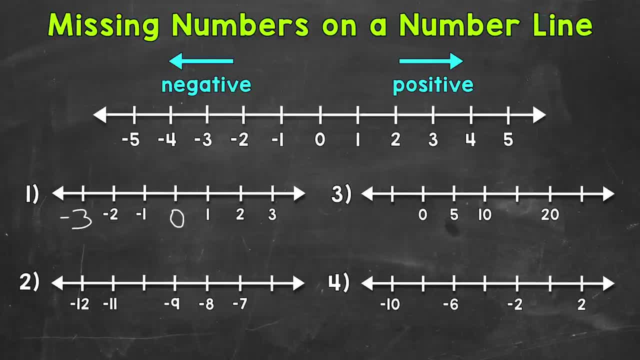 Let's see if that applies to the rest of the number line. So we have negative nine, negative eight, negative seven, So we can tell that we're counting by one. So let's start at negative twelve and count up by one in order to find these missing numbers. 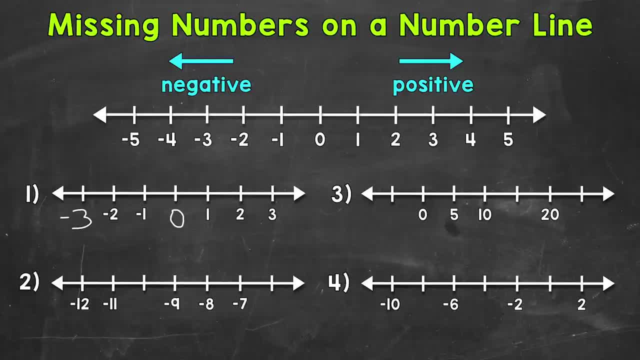 Negative twelve, negative eleven. then we have negative ten, So that's our first missing number. Then we have negative nine, negative eight, negative seven and then negative six for our other missing number. And we can always double check by counting up or down and seeing if those missing numbers are correct. 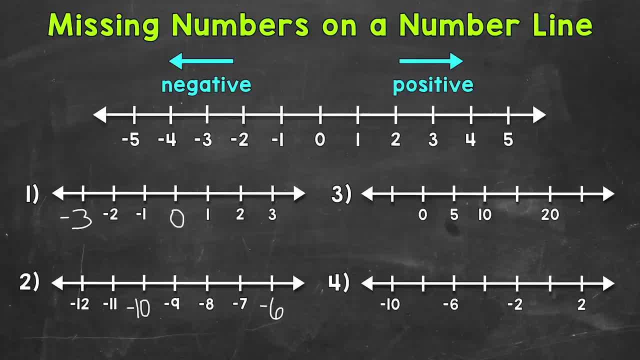 So let's count down Negative six negative seven. negative eight. negative nine, negative ten negative eleven and negative twelve. So those missing numbers fit in that number line. Let's move on to number three, where we have a missing number to start off with. 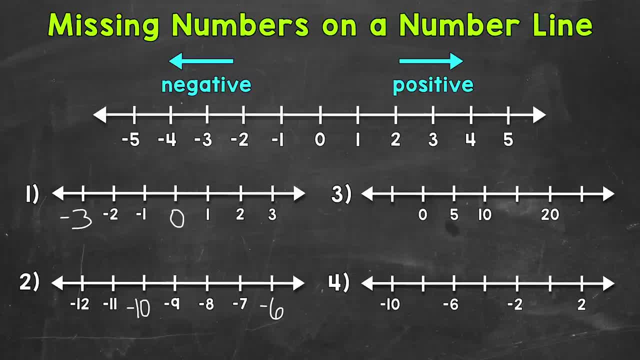 Then we have zero five, ten, a missing number, twenty, and then another missing number. So let's take a look at what we're given: Zero five, ten. So the distance between those numbers that we are given is five. 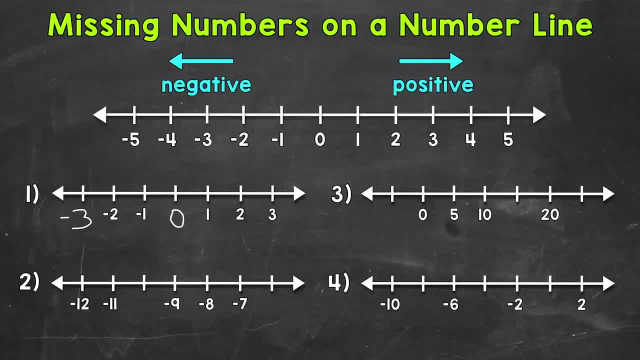 Let's see if that applies to the rest of the number line. So we have negative nine, negative eight, negative seven, So we can tell that we're counting by one. So let's start at negative twelve and count up by one in order to find these missing numbers. 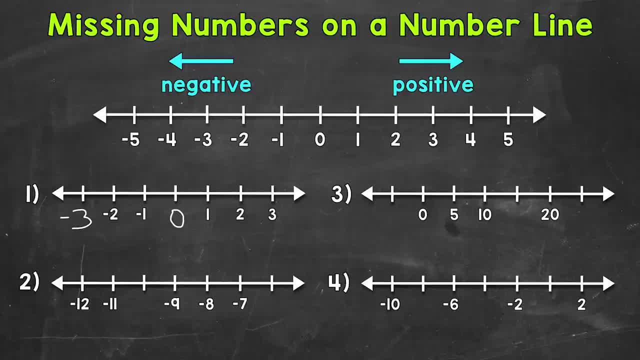 Negative twelve, negative eleven. then we have negative ten, So that's our first missing number. Then we have negative nine, negative eight, negative seven and then negative six for our other missing number. And we can always double check by counting up or down and seeing if those missing numbers are correct. 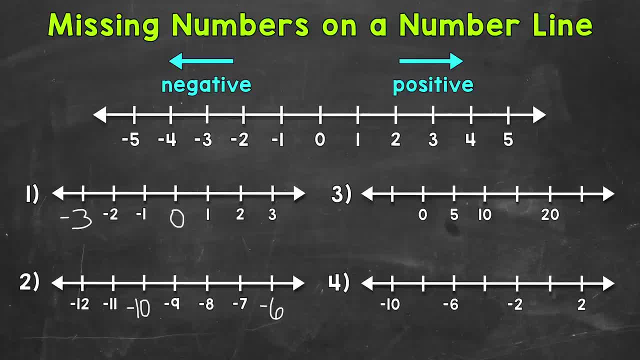 So let's count down Negative six negative seven. negative eight. negative nine, negative ten negative eleven and negative twelve. So those missing numbers fit in that number line. Let's move on to number three, where we have a missing number to start off with. 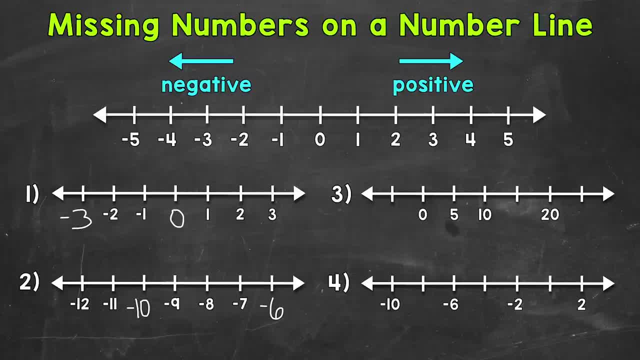 Then we have zero, five, ten, a missing number, twenty and then another missing number. So let's take a look at what we're given: 0, 5, 10. so the distance between those numbers that we are given is 5, so it looks like we're counting. 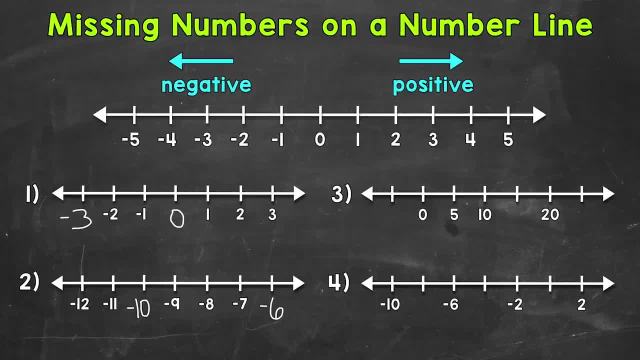 So it looks like we're counting up by five. So let's do zero, five, ten and then fill in that missing number between ten and twenty first. Now it doesn't matter what order you fill in the missing numbers. There are different ways to go about this. 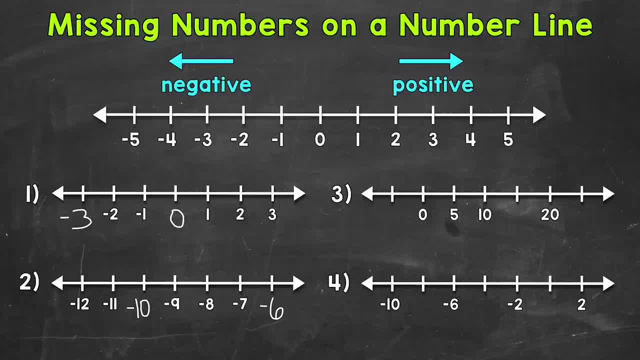 I'm giving you some strategies that you can use in order to fill in these missing numbers. So whatever works best for you. So zero, five, ten, Then we have fifteen. So again we're counting by five here. Then we have twenty. 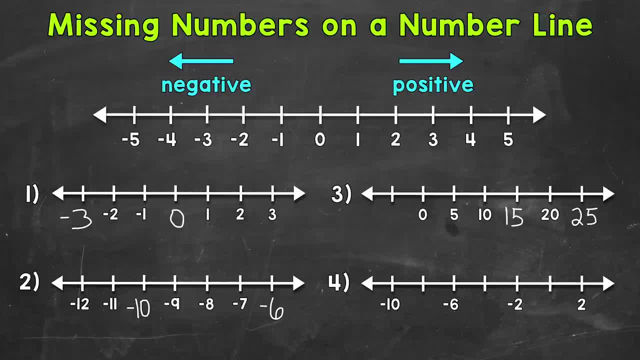 And then twenty-five. Now we need to go left on our number line, decrease in value and count down. So let's start from twenty-five and go all the way through and then fill in that missing number. So twenty-five, twenty fifteen, ten, five, zero. 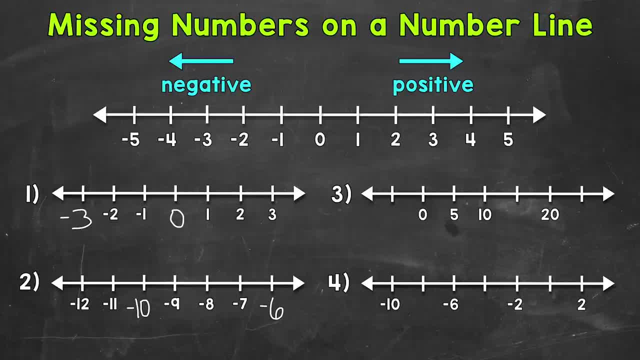 up by 5. so let's do 0, 5, 10 and then fill in that missing number between 10 and 20 first. now it doesn't matter what order you fill in the missing numbers. there are different ways to go about this. i'm giving you some strategies that you can use in order to fill in these missing numbers. so 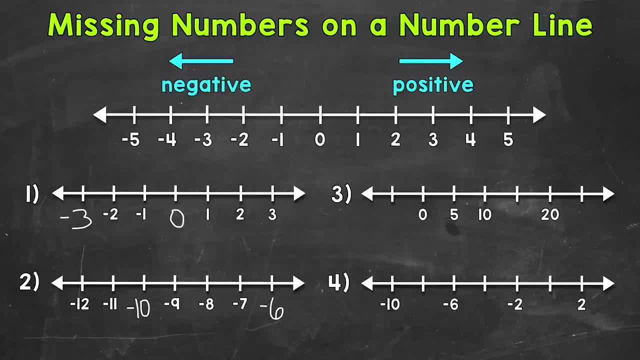 whatever works best for you. so 0, 5, 10, then we have 15. so again we're counting by 5 here. then we have 20 and then 25. now we need to go left on our number line, decrease in value and count down. so let's start from 25 and go all the way through and then fill in that missing. 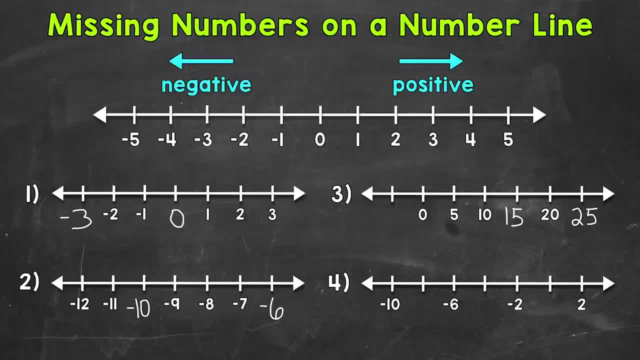 number. so 25, 20, 15, 10, 15, 0 and then negative 5. so for that one we were counting by 5. lastly, we have number 4, and for this one we don't have any consecutive numbers, meaning we don't have any numbers on this number. 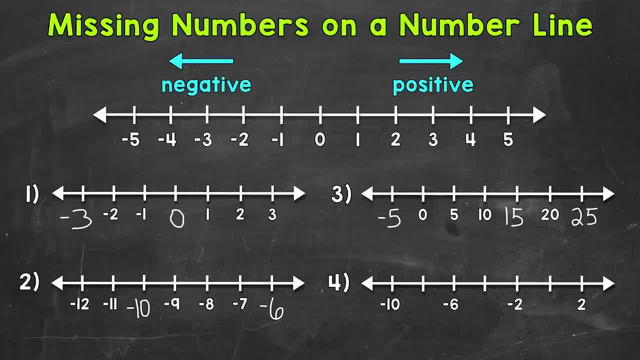 line next to each other, but we can still use what we're given. so we have negative 10, a missing number, negative 6, a missing number, negative 2, a missing number, and then 2- let's start in between negative 10 and negative 6, so we have a distance of 4 between those two numbers. well, 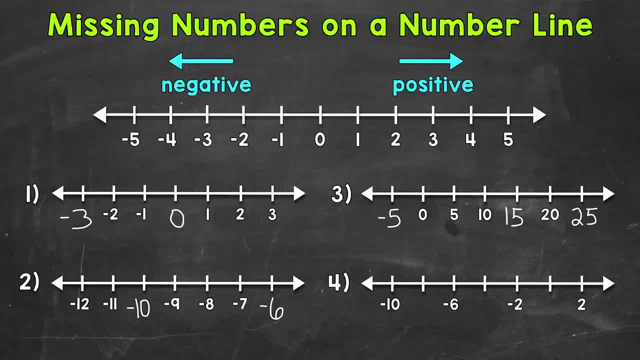 what's going to be directly in between negative 10 and negative 6? well, negative 8. so negative 8 goes here and we have negative 10, negative 8, negative 6. it looks like the distance between numbers on this number line is 2, so we are counting by 2, so our next missing number: 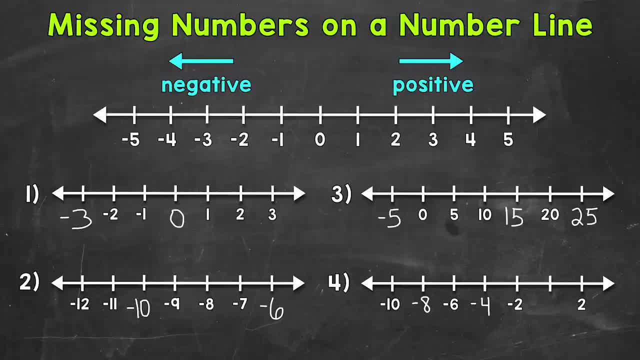 is going to be negative 4, then we have negative 2 and then 0 and then a positive 2, so we were able to use what we were given there, even though we didn't have consecutive numbers- meaning numbers next to each other- and fill in those missing numbers. you can almost think of these. 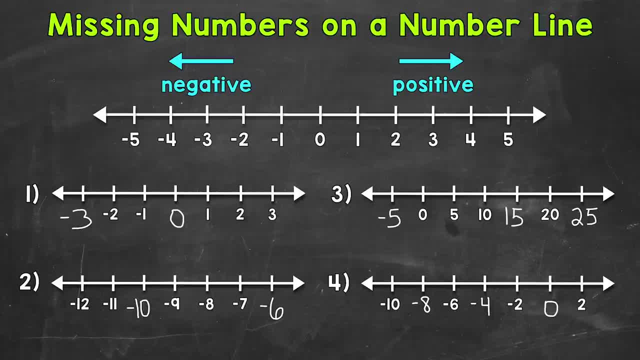 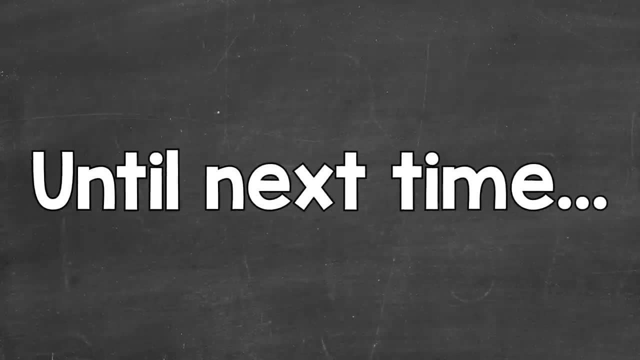 like filling in a pattern. we need to find that distance between the numbers on the number line, so the intervals, and then apply that to the missing numbers counting up or counting down. so I hope that helped. thanks so much for watching. until next time, peace.